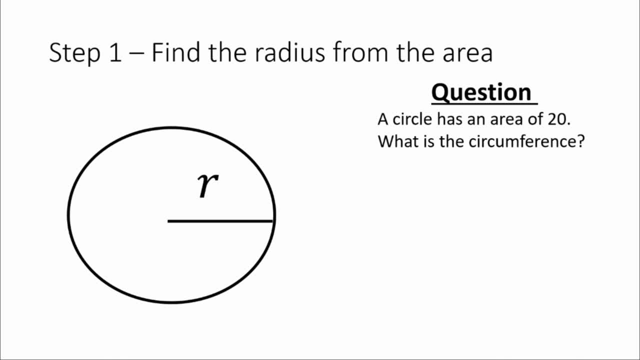 radius from the area. So in order to get the circumference, we have to first have the radius, because that's going to be the link. So what we need to do first is recall the equation for the area of a circle, which is that the area is equal to pi multiplied by r squared. We want to get the. 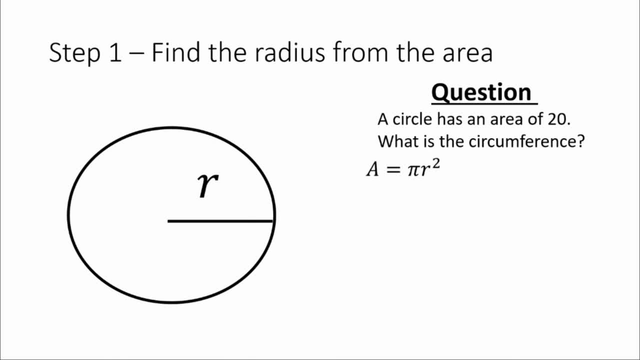 radius. so this equation needs to be rearranged for the radius. So we start by rearranging by dividing both sides by pi, which gives us this expression: We don't want r squared, we want r, so we need to square root both sides so we get that the radius is equal to the square root of. 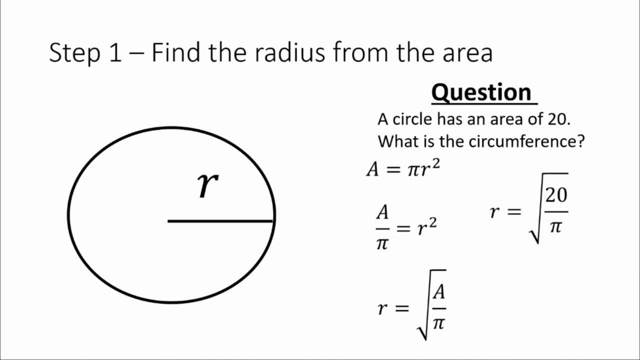 the area divided by pi. So our area, we're told in the question, is 20.. So we're going to do the square root of 20 over pi. You put that into a calculator Carefully and evaluate it and you get 2.52. when rounded to two decimal places You could leave. 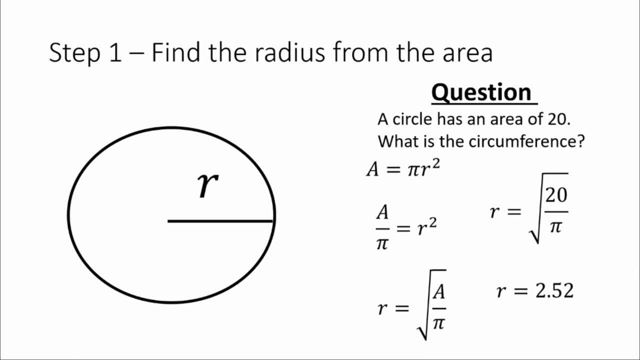 that as an exact value, though for this video I'm going to keep everything to two decimal places. We then need to look at the second step, which is to find the circumference from the radius. So, again, we need to take forward our previous answers and recall an important equation. So, 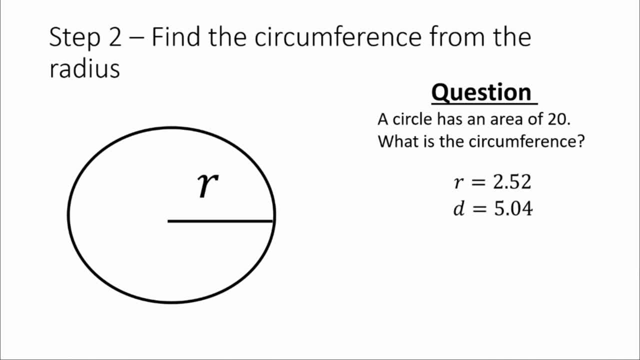 we've got, the radius is 2.52 that we just calculated. That means that the diameter is going to be double that. So again, working in two decimal places, We just double that value and we get the diameter to be 5.04.. We then know that the circumference 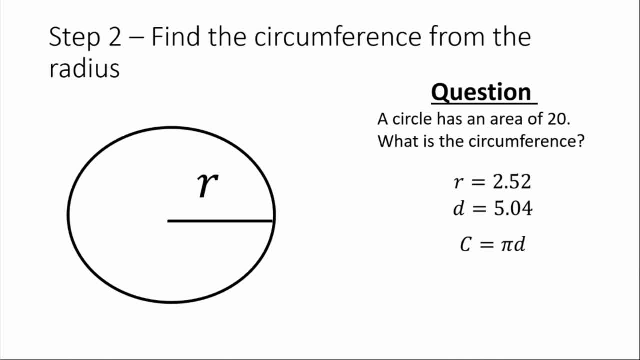 is the diameter multiplied by pi. So we can use that equation. So all we have to do is just put in our diameter. So we've got the circumference is 5.04 pi, and if you wanted to get that as a decimal rather than as an exact value multiplied by pi, you would just put that in a calculator and you 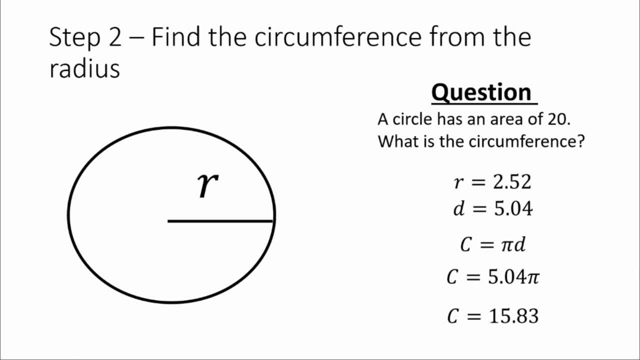 would get 15.83 again to two decimal places. I hope this video was helpful to you and you know the two simple steps that let you go from area to circumference. If this video was helpful, please like and subscribe below and finally, thank you very much for watching.